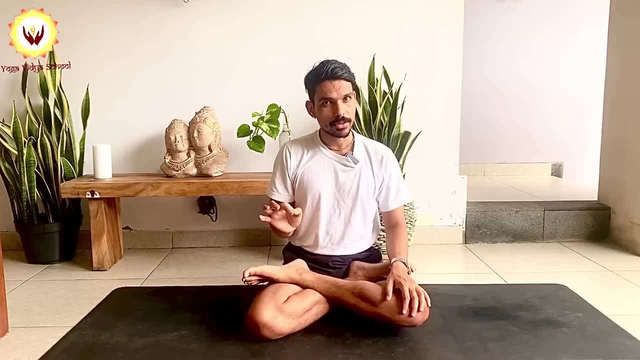 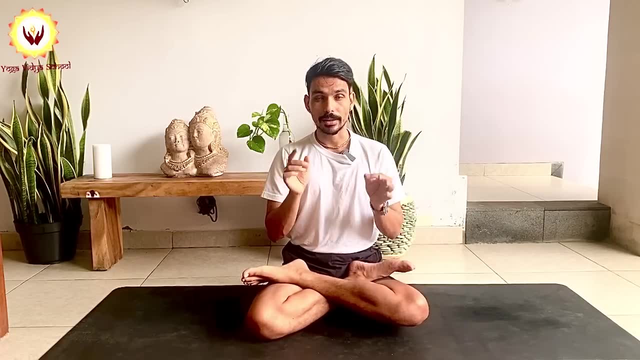 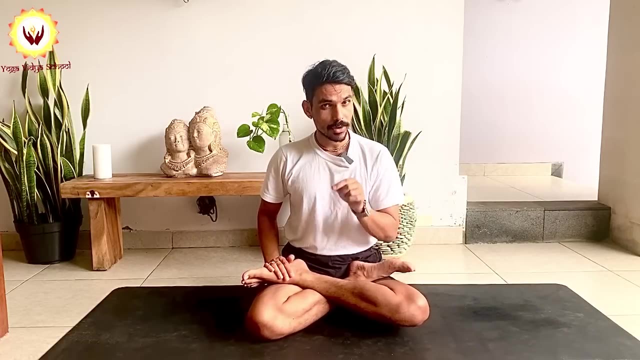 and also it helps to convert the sexual energy into spiritual development. So those who really want spiritual growth, who really want their consciousness to expand, this asana is very important. You must start this asana from today. only In today's class, I am going to teach you what is Siddhasana, how to perform right way. 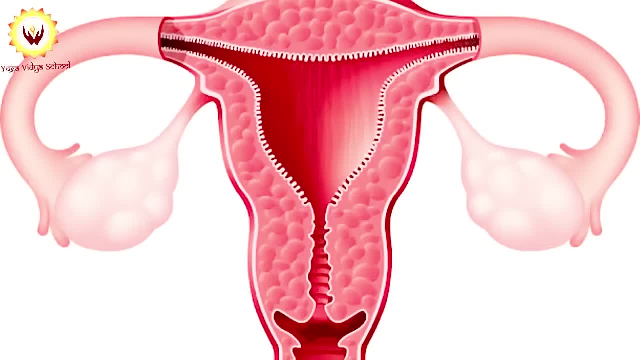 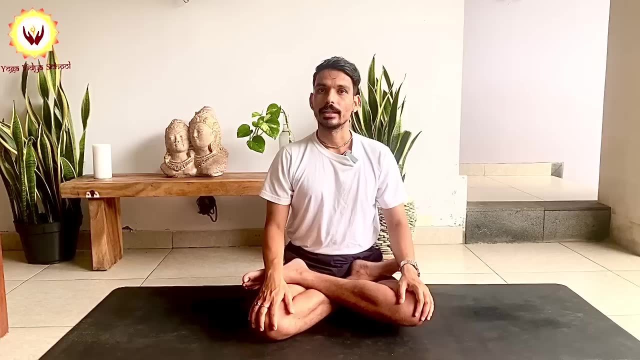 which can help you physically, which can improve the health of reproductive organs and the disease problems related to these reproductive areas. Let's begin the practice. And those who wants to start their yogic practice with me every morning, 6.30 am, I am giving live. 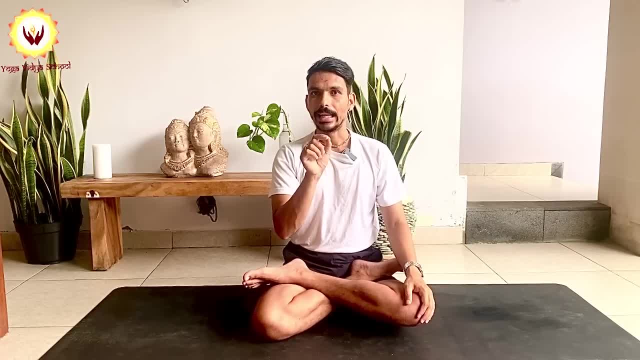 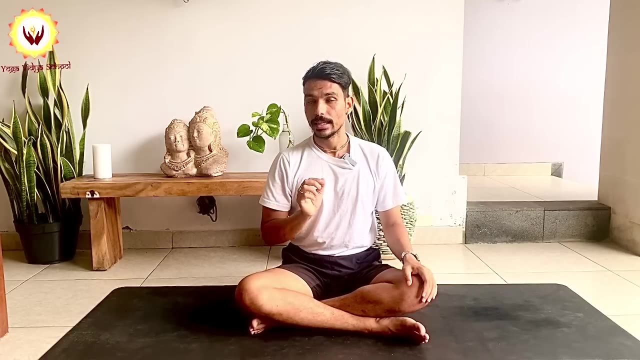 classes on zoom. So those who are interested link in description the detail and the contact number. You can go and enquire there. Next month you can start your yogic practices every morning and make yourself healthy and happy. So for Siddhasana there are few confusion. Some say that use the right leg first in the 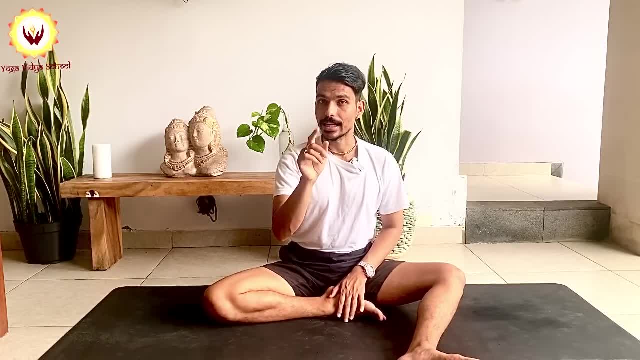 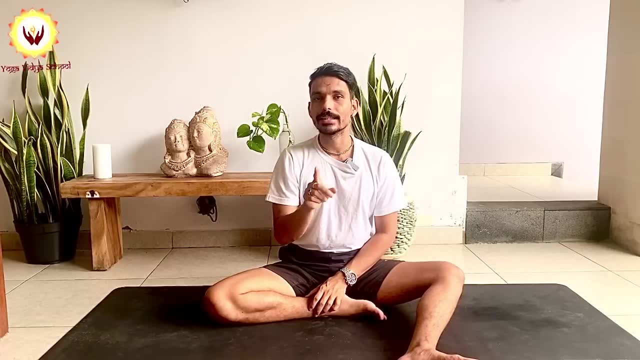 bottom, Because Siddhasana what it does. Siddhasana controls the Vajranadi. We have 72,000 energy channels and these all energy channels can be purified by Siddhasana because by doing this asana, the force of apana moves. 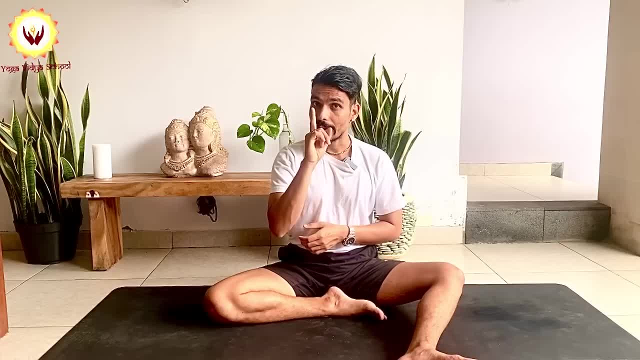 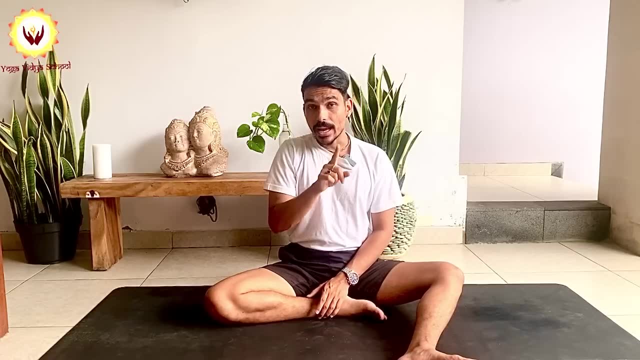 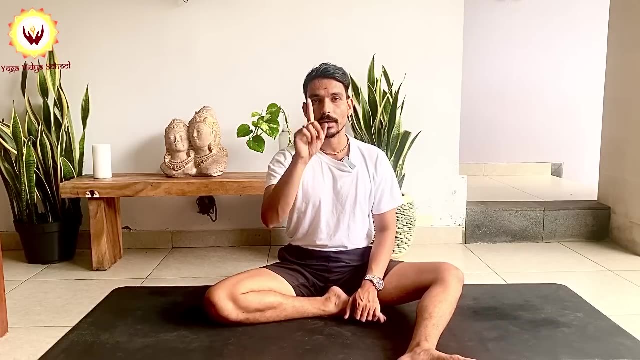 Asana moves upward direction. This asana helps the apanavayu to channelize upward, to the sahasrara, and this is how the desires converts into liberation. One of the energy channel is named as Vajranadi, which is responsible for apanavayu harmonization and which is also responsible 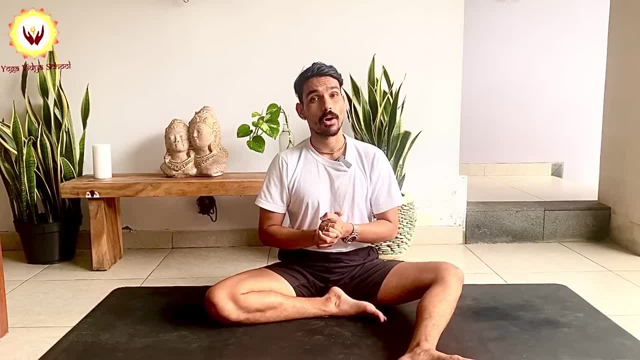 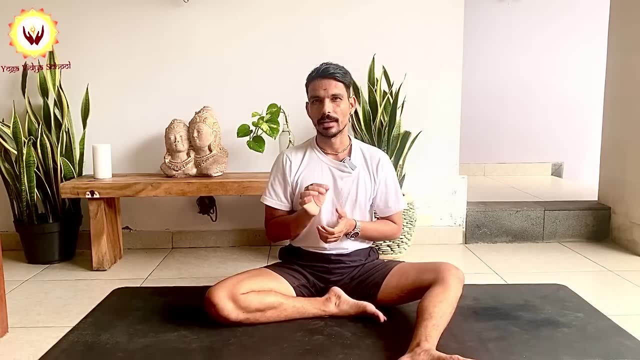 for reproductive area control. The function of reproductive organs is controlled and managed by this particular nadi, So those who are interested click on the link in description If you are having any problem related to reproductive area, for example too much desire sexual. 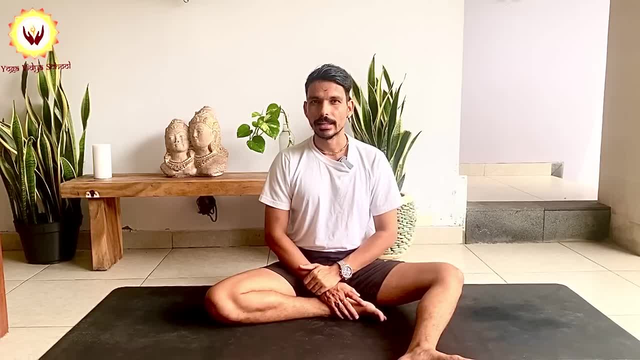 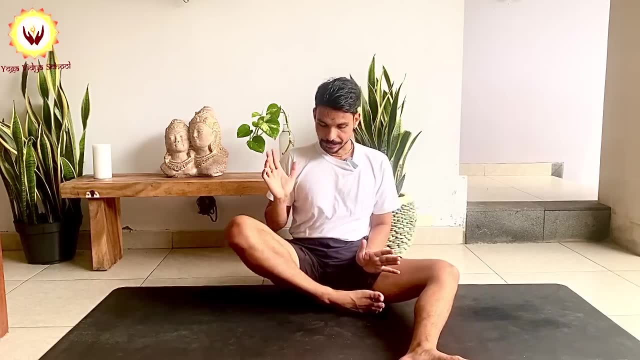 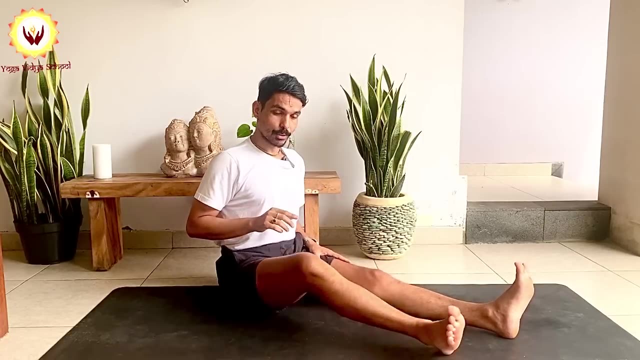 energy is not managed, not controlled, so to change it, this asana is very helpful. So the right leg first see here. So this is sitting asana, so you must stay first dandasana. When you stay in dandasana, I would request you to first drop the leg, like this: 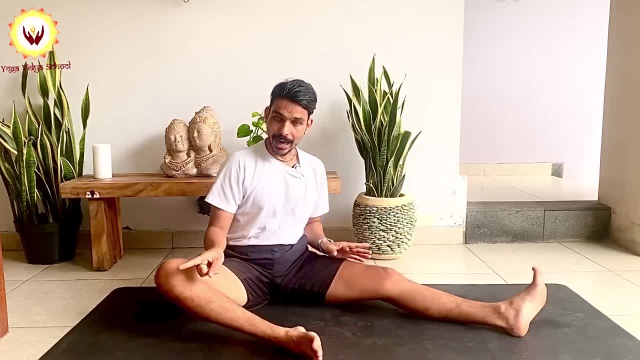 what we learn in padamasana: You just drop- Take this knee up. you just drop the leg like this. You just drop the leg like this. You just drop the leg like this. You just drop this leg like this. You just drop this leg like this. You just drop this leg like this. 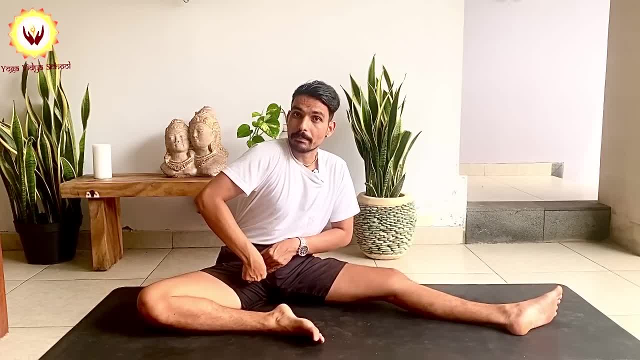 bli estamosавçam saider or pac divina celرة. 28 And diferentesvem controversiali elderly personii codave pau, The heart is here. It is here, It is called meditatory. oursi ceaa Siddha ask braking Kalsi. 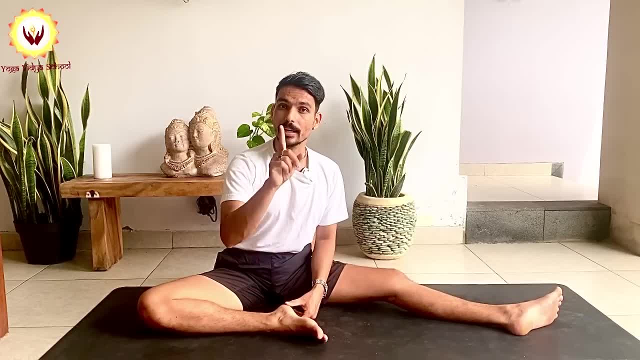 Siddha sank GC kat quiš妳 tr chats. If you are out, that means you are shut As much as possible. until you are not opening the pelvic region, you will not be able to do siddhasana. The way to work is done. 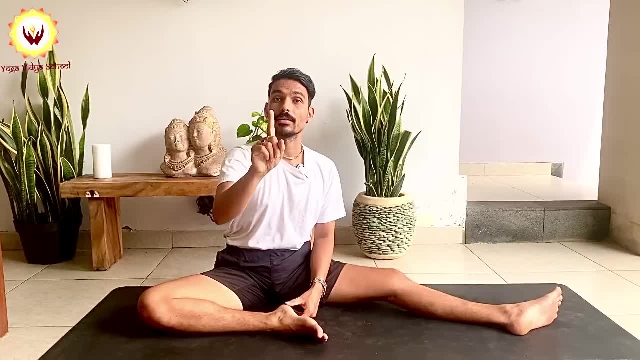 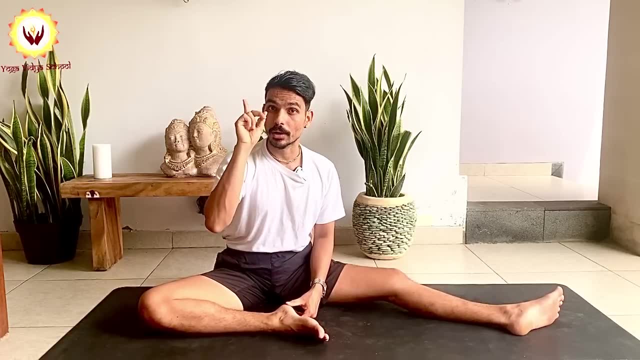 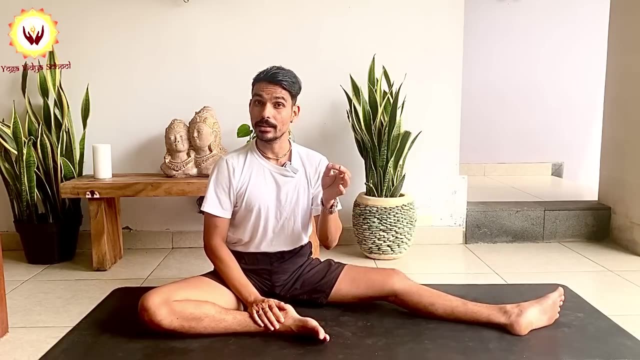 When the pranic flow is channelizing upward direction. this is called sitt. and the person who can channelize that prana not downward but upward direction, for the spiritual growth, for the full development of the mind, this is called siddha purusha. siddha person means: 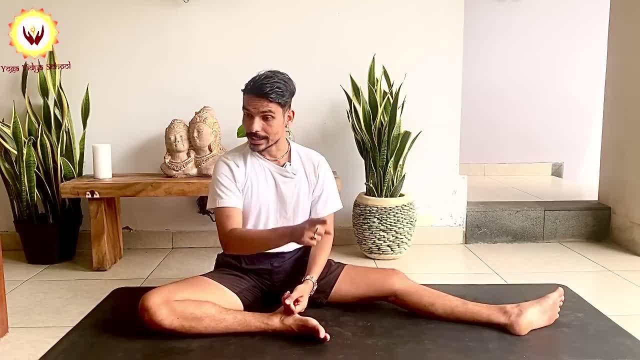 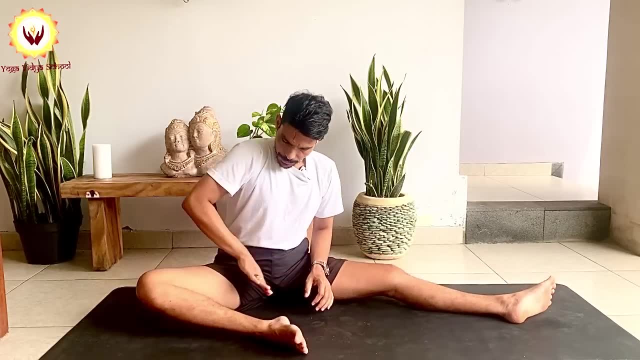 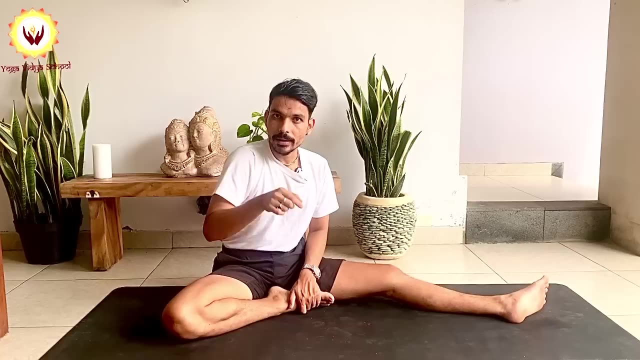 the person who convert the flow of prana, Not for the desire brait, for the desire condition, for the desire, but for the spiritual growth, for the enlightenment. understand. so first you take your knee out as much as possible now right heel will be placed between the reproductive organ and. 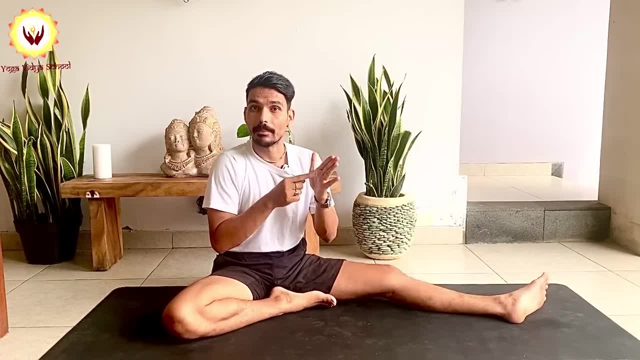 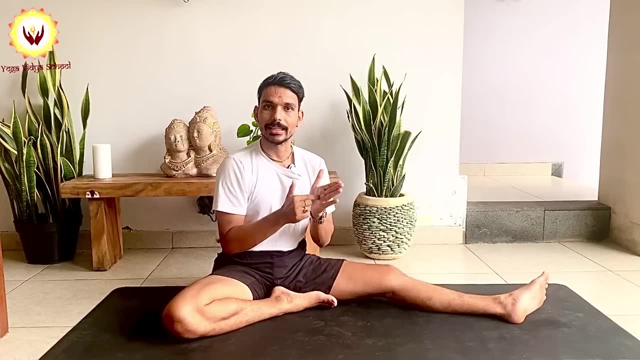 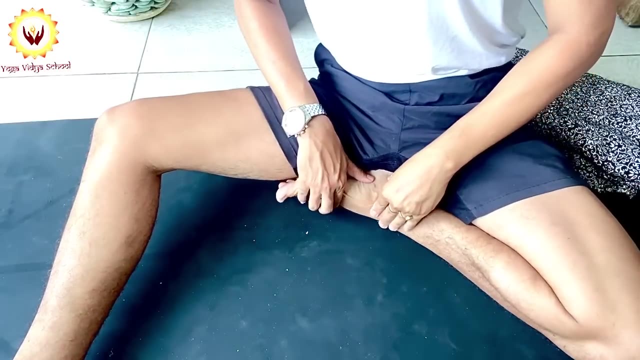 the anus door. this is the area of mooladhara, between the anus and the testicle in the male body reproductive area and the anus, between that that area. so you will press here, so you can see that this area, when you press that area, you will feel little pressure into that particular space. 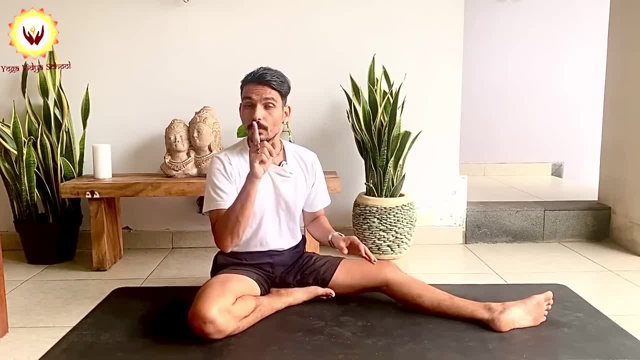 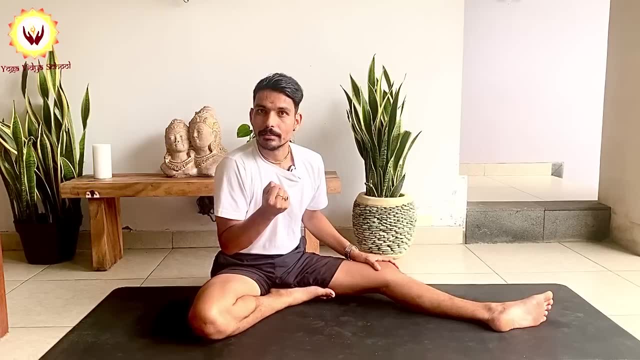 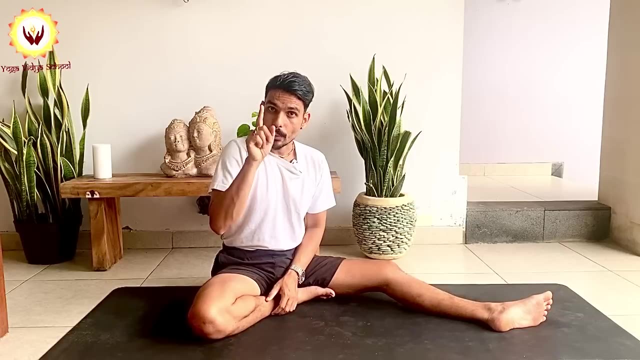 and that pressure is important because when you press, this mooladhara is stimulated and this energy center, mooladhara, is responsible for this Kundalini Shakti. mooladhara is a generator of energy system, means you generate the prana from there. so when you press with your heel and many 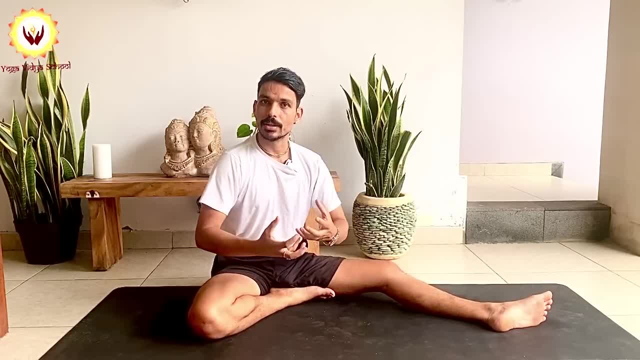 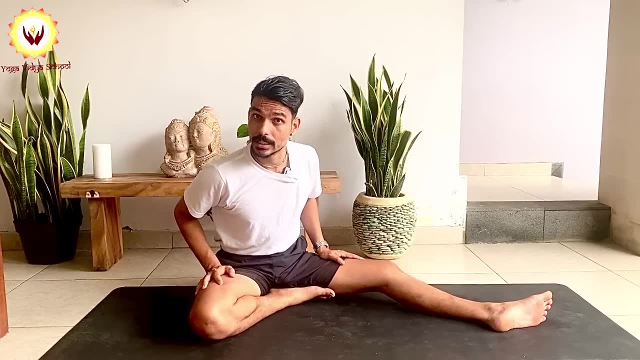 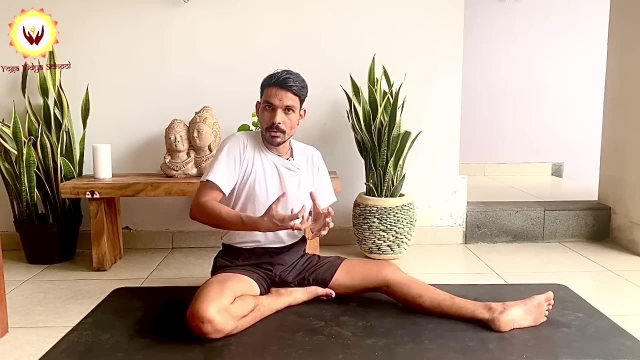 constant giving pressure. so the energy, the prana, is generating slowly, slowly, slowly, and you can feel the heat, even the lower part of the body. after 15 minutes of sitting in siddhasana you can feel that the lower body completely in burning sensation. everyone can feel that it means now the flow is generated. it's like 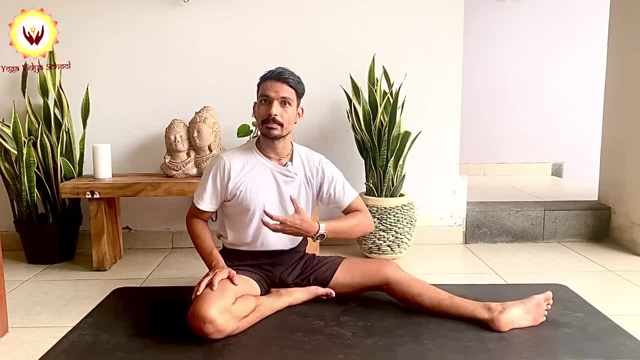 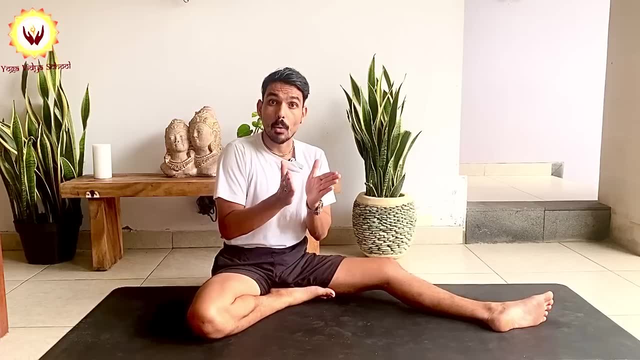 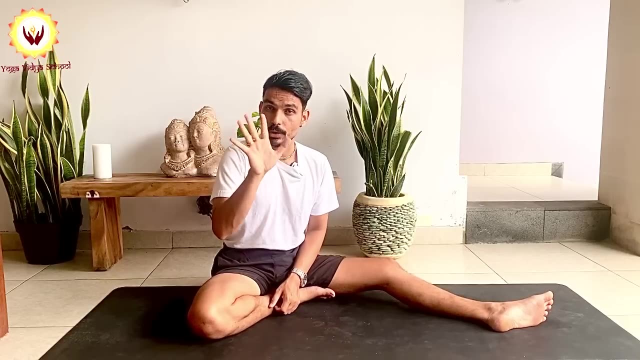 when there's no power, you open the generator. how generator produce the energy? similarly, when you press the heel, it produce the energy more and more and muladhara door is start opening, from through which the energy start moving upwards, slowly, slowly, with gentle pulsation, which you can. 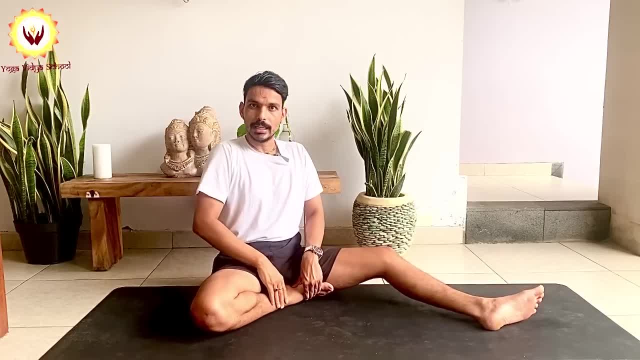 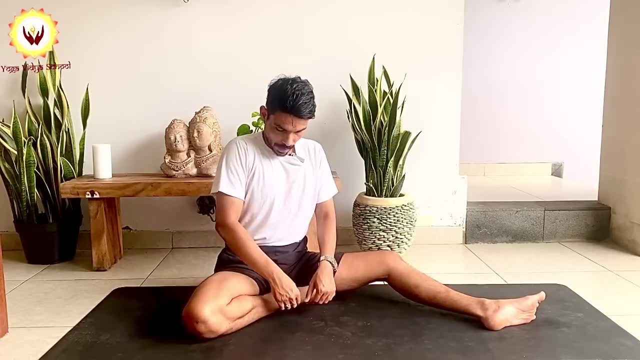 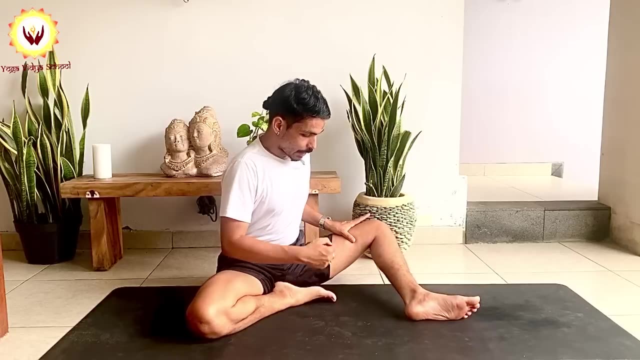 experience when you perform this asana. so first is placing the heel, the right heel, there and see this area between the calf and the thigh completely closed. so i'm just giving pressure, tilting the buttock little forward now this leg, so you open this leg also to the sideways. 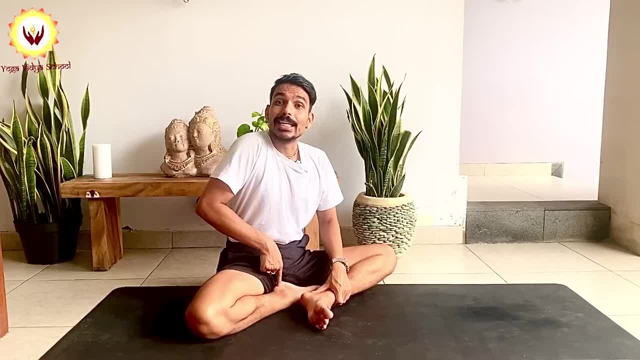 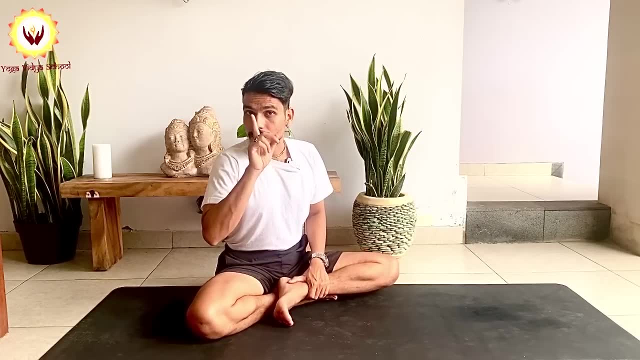 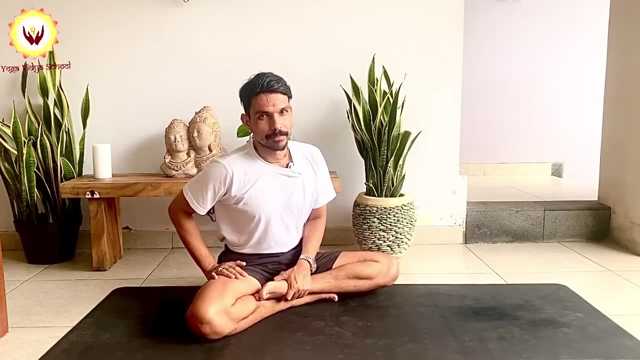 and this heel will come top of the right heel. the left heel will come top of the right heel, like that. here now the question come. books and scriptures says how to perform right way when the heel will come on the top for the male body, this heel, the left. 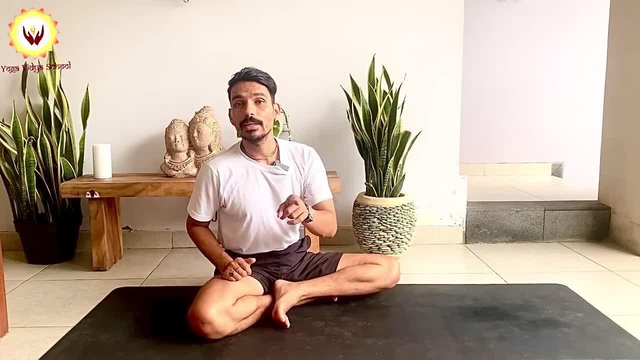 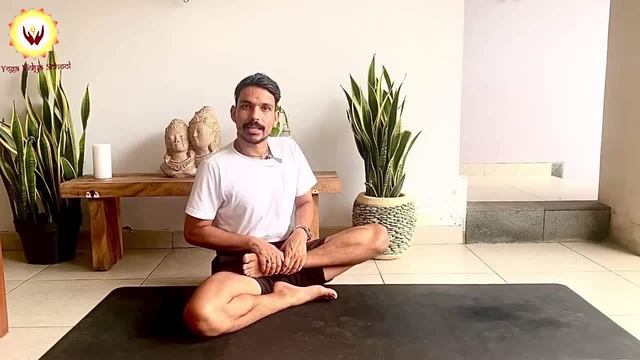 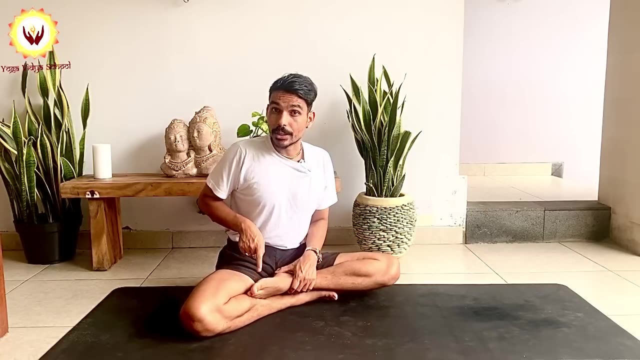 heel which is above that hill, should be above the penis area, the root of the penis. so the root of the penis, this heel will be on the top of this and when you so, it means the penis will come between. and then you press the, the toes, and push this toes between the calf and the. 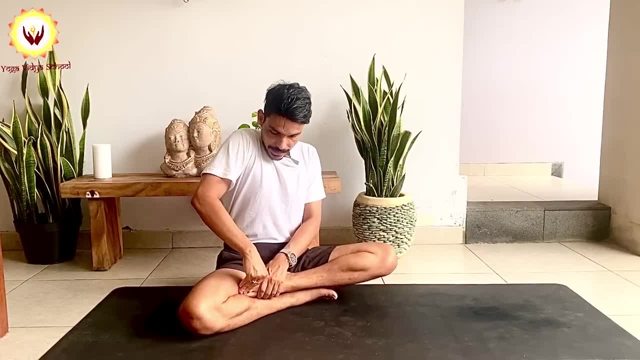 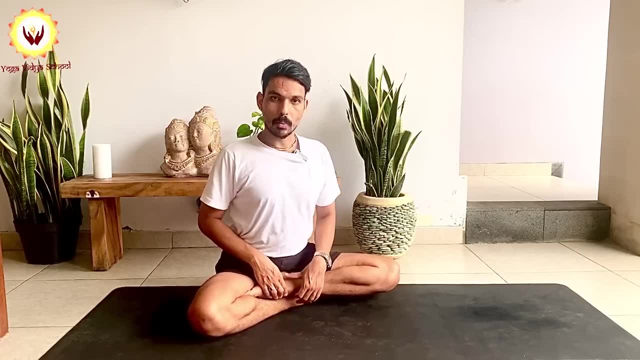 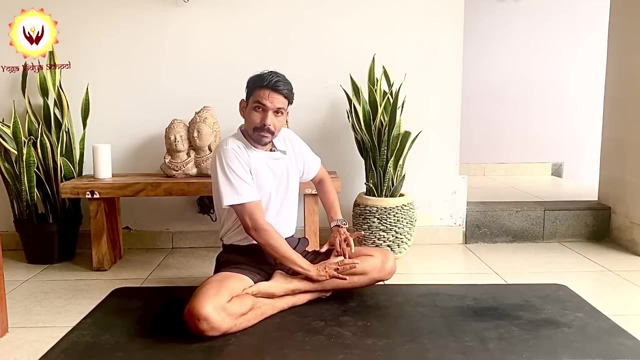 thigh of the right leg. so see, here i will start pressing this down, down, down, down, and then it's locked heel to my swadhisthana center, here and now. what about the lower foot? so now you need to open the gap between the calf and the thigh of the left leg and then start bringing the 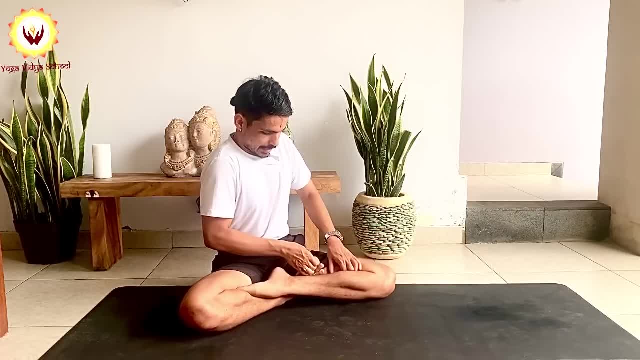 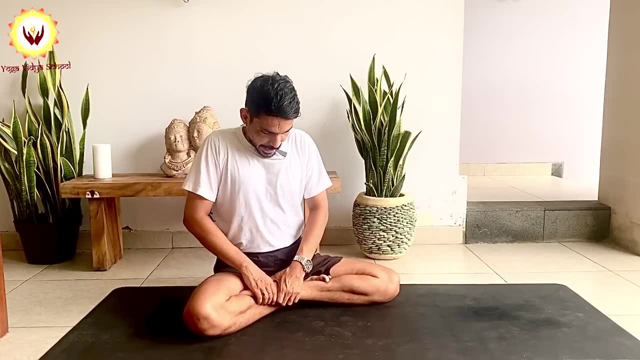 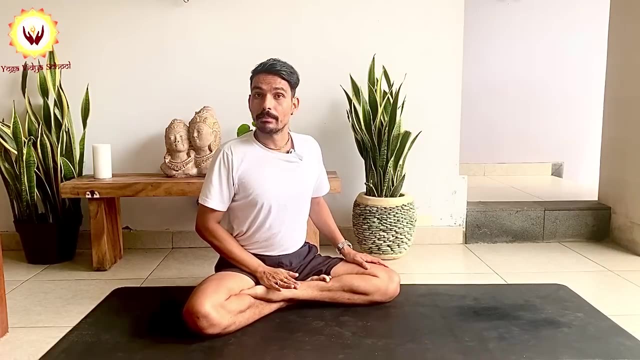 right toes, right toes up, up. see here, this is how it has to be. so this left toes will slightly go down and the right toes will come up and heel will be the left heel above heel will be above the penis, in the male, in the female it will be the same way- above the vaginal area and then these: 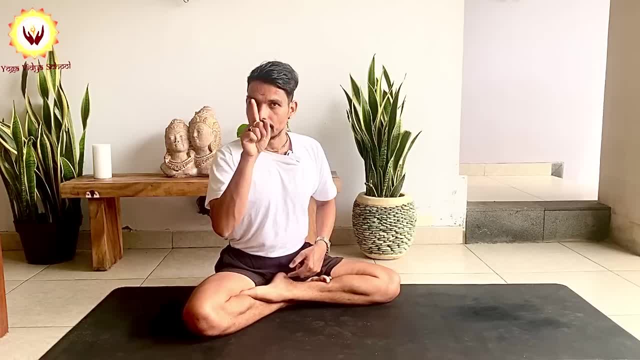 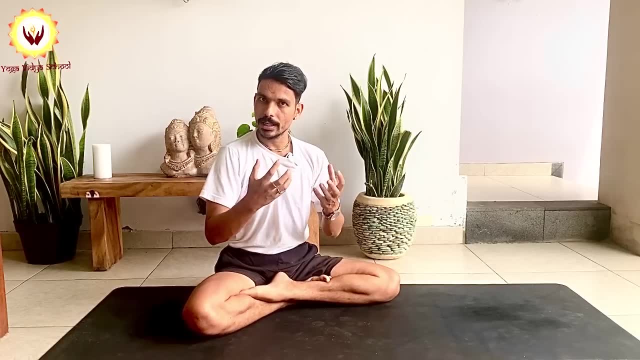 two heels will press these two particular points. the bottom heel will press the mooladhara point, from where the pulsation will start. from where the pulsation will start, the generator will start, the energy will generate, and this is the area of swadhisthana and in this area the channelization will start. 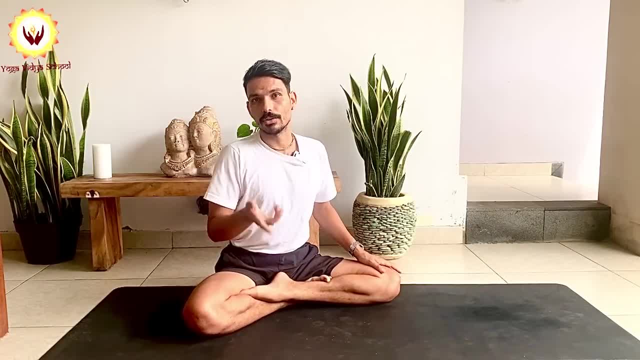 so from mooladhara you generate and from swadhisthana pressure you channelize, in this position what happens? spine becomes straight. there are four asana in which the spine becomes completely straight, which i mentioned earlier: simhasana, padmasana, siddhasana. 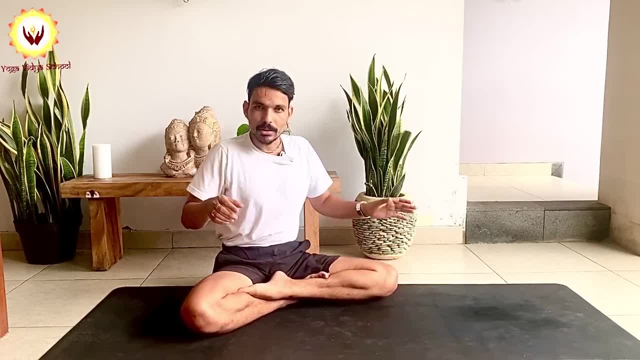 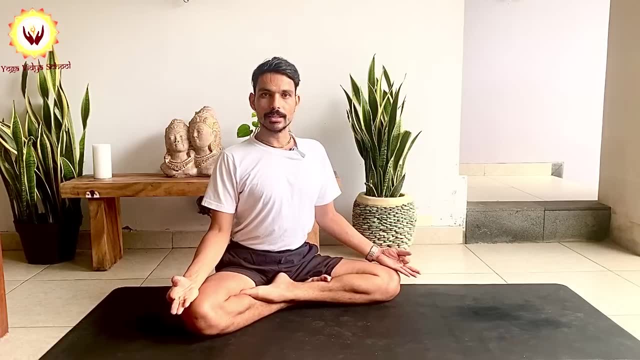 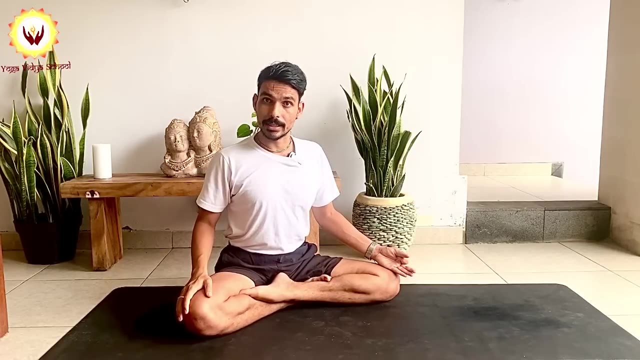 and bhadrasana. so in this asana your spine is not curved because you are tilting forward. this is how, and then you can do any hast mudra, either chin or gyan. mudra this and stay with closed eyes, focus in this particular two points and then do meditation for 15 minutes every day. 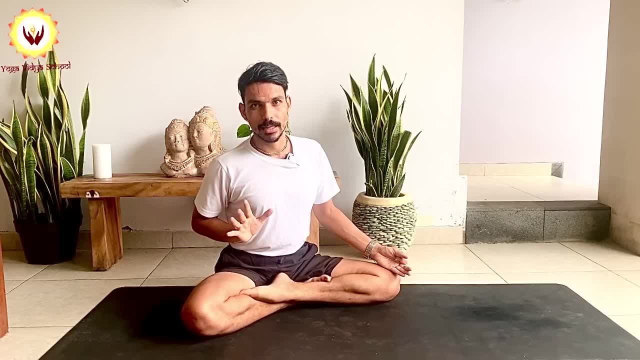 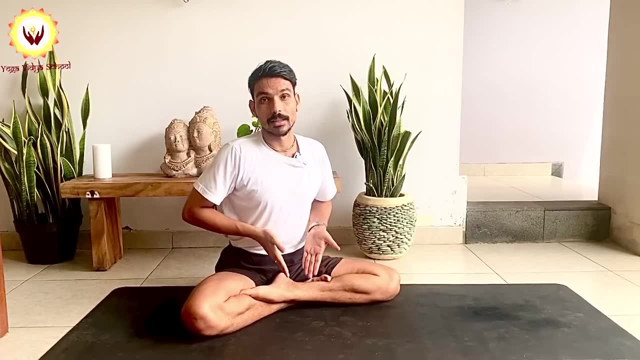 it will solve all your reproductive related problems. spiritual development: this asana is very beneficial for pranayama practice. two asana you must use: padmasana and siddhasana meditation. padmasana and siddhasana: you will grow fast in your spiritual journey. 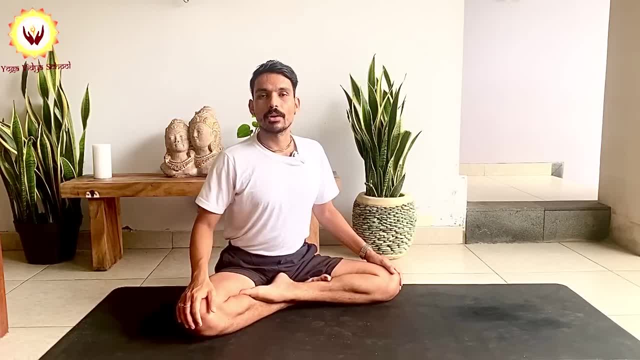 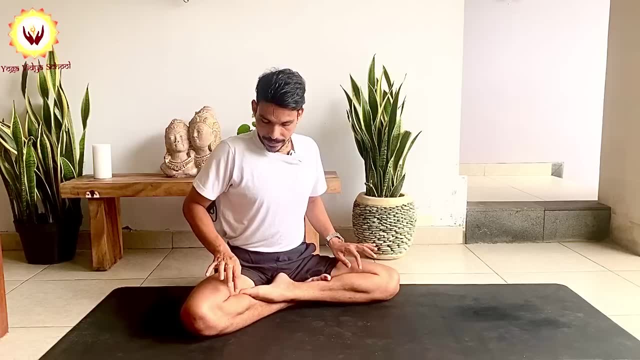 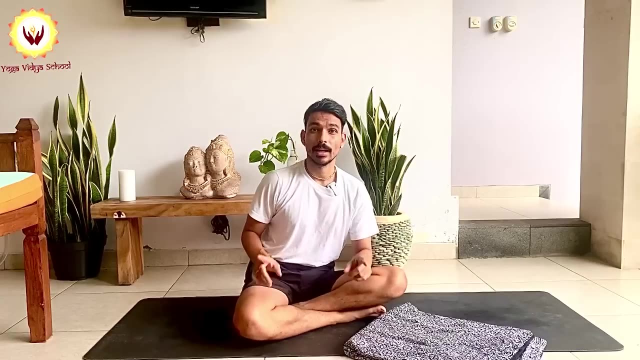 this asana is not very easy pose, so for beginners it will be quite challenging. because for beginners you will feel pain on the ankle, you will feel pain here, your spine will curve. so i would suggest to use the folded blanket for few times. see here, i will fold the blanket like that and i will place. 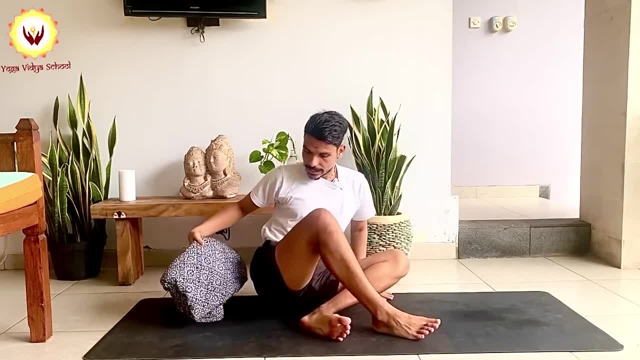 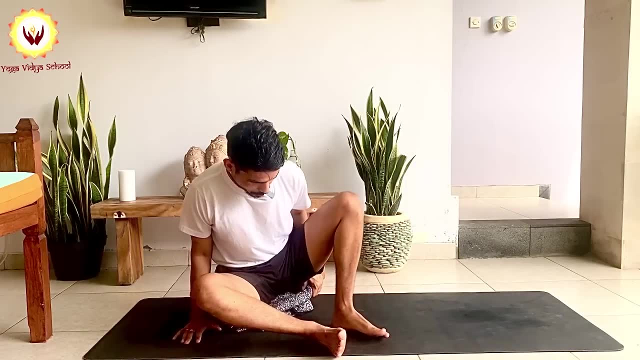 it under my buttocks and then it will be easier to perform siddhasana. again, i will show you, and then i will show you how to do the siddhasana. again i will show you, and this time i will show you from the left. now the question is: start from the left or right? 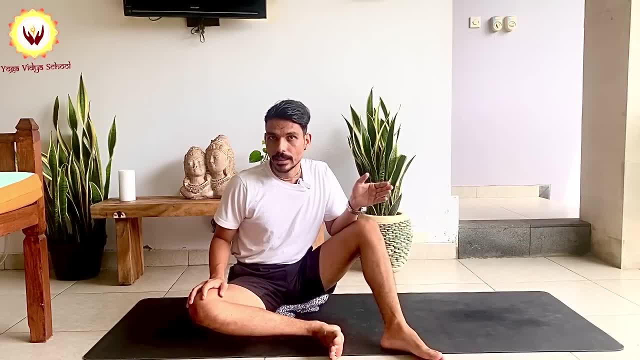 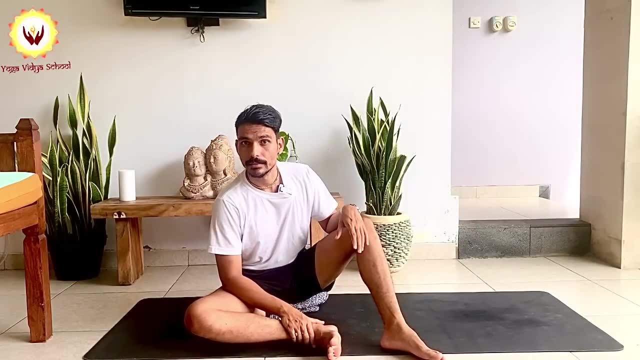 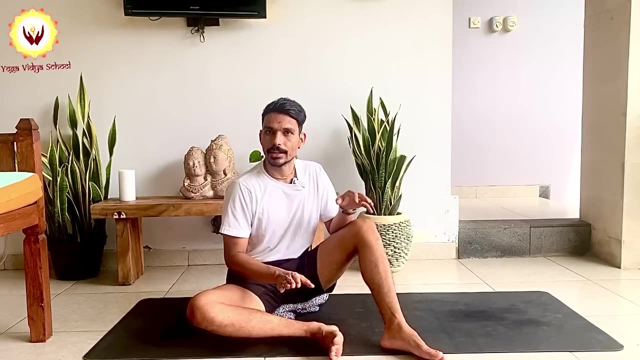 see, according to the scriptures, many scriptures which was written in past time says the right heel will come first, but some people they cannot do with right, so you can do left also first, because many different yogis they have experienced with the different legs, because there are two types of 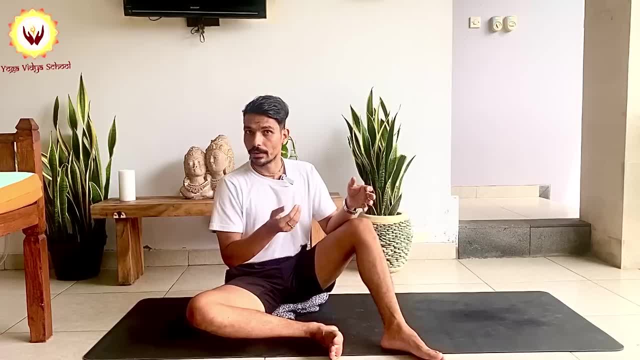 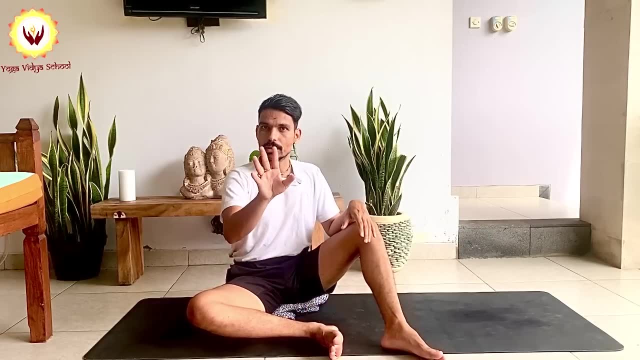 knowledge. one knowledge which comes from the scripture- you read the scripture, you learn- and one comes by the guru parampara, the lineage, some traditions says the left down, some says right, you start, which is more comfortable, because some people they can do right first, easier, some people cannot, so you choose. 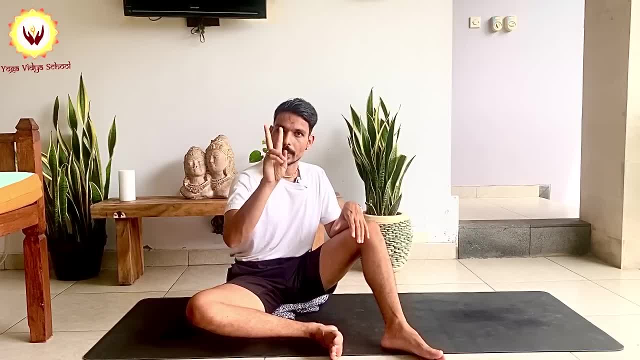 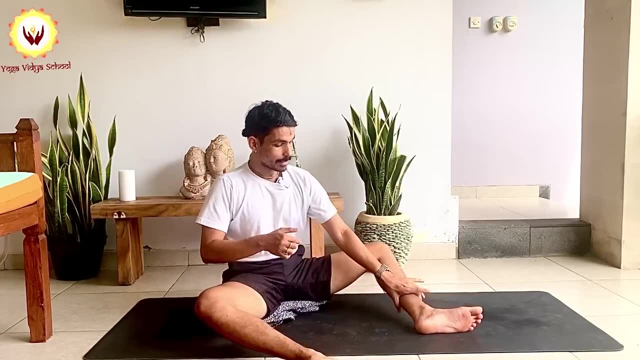 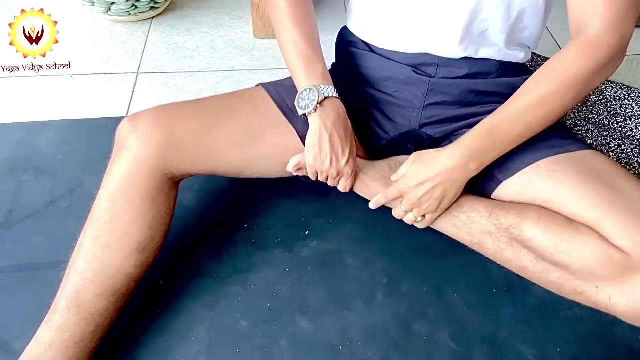 your which is more comfortable for you. but the main is two, two points and the pressure. this is important. let me show you now from the left side. so first i will drop the leg outside, i will take this backward as back as possible, and now i will bring this heel there between the anus and the